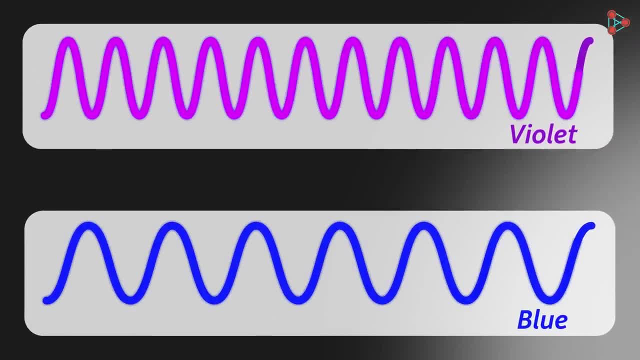 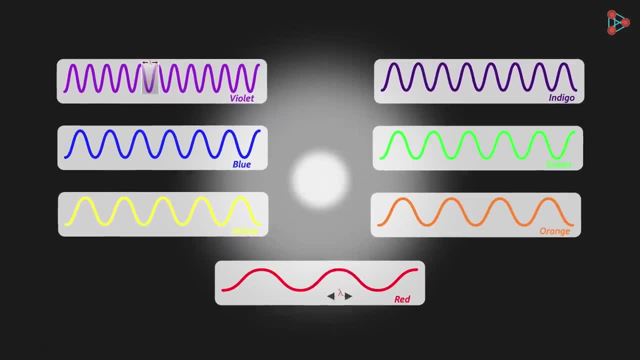 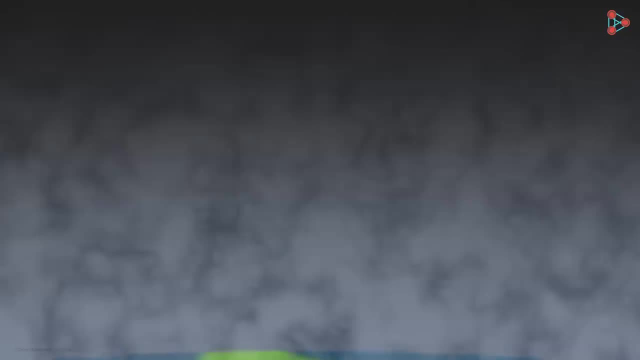 and each coloured light has a corresponding frequency and wavelength associated with it. The violet coloured light has the shortest wavelength of all, while the red one has the largest wavelength. And what forms the earth's atmosphere? The earth's atmosphere is mainly composed of gases, dust, particles, water droplets and water vapour. 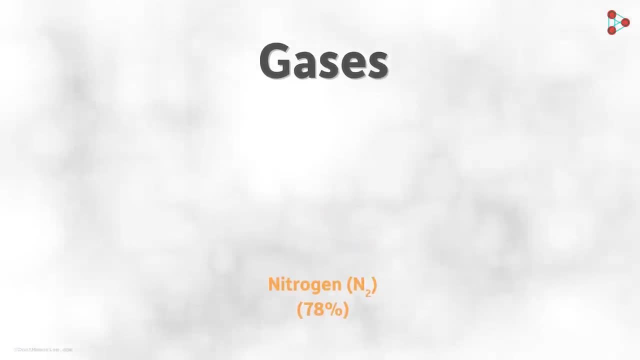 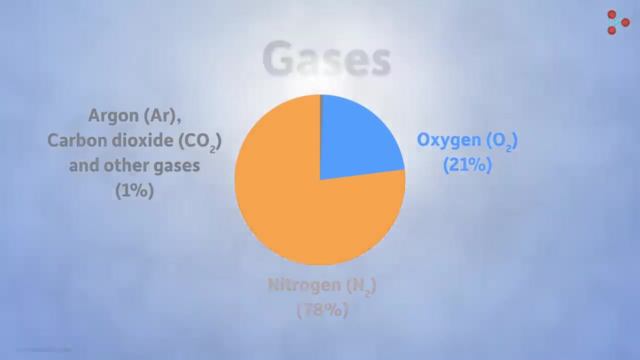 Among the gases, nitrogen is present in abundant quantity, at around 78%. It is followed by oxygen, which is approximately 21%, and the remaining is filled with the likes of argon, carbon dioxide and other gases. First, let's see what happens when the sunlight falls on these air molecules. 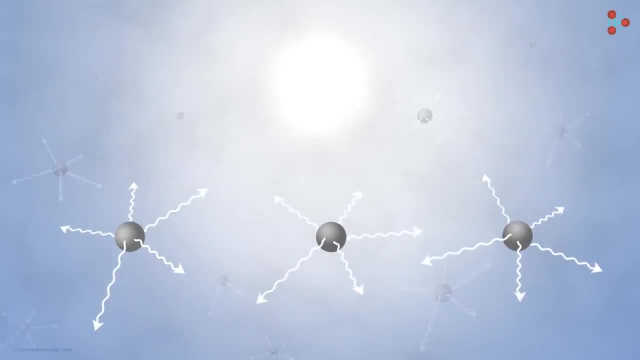 When sunlight falls on these air molecules, the atmosphere is filled with oxygen. When sunlight falls on these air molecules, the atmosphere is filled with oxygen. light strikes these molecules. it gets scattered. Scattering is a process in which the light is absorbed by the atoms and re-emitted back in various directions. However, not all the 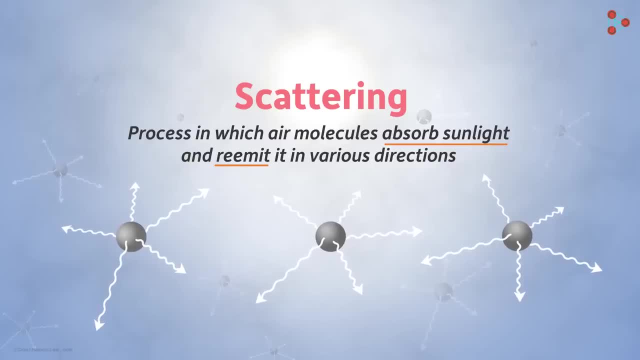 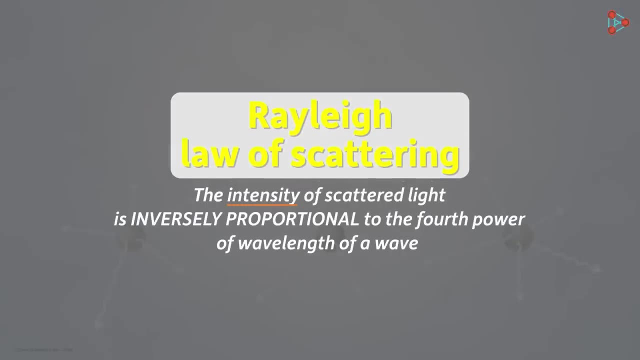 light is scattered. equally, The amount of light that will be scattered is given by the Rayleigh law of scattering. It says that the amount of scattered light, or the intensity of the scattered light, is inversely proportional to the fourth power of the wavelength of a. 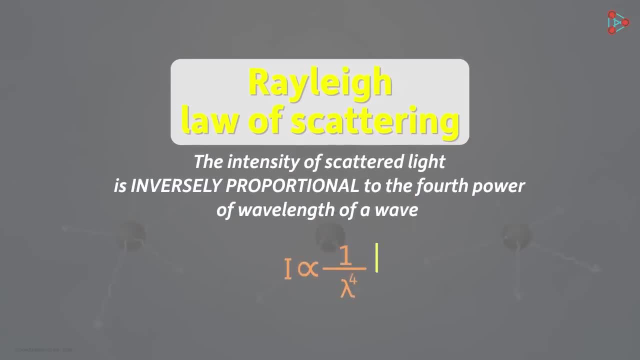 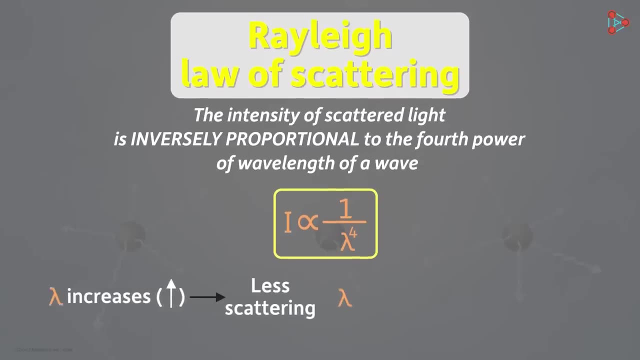 wave I is inversely proportional to lambda, to the fourth power. If the value of lambda increases, then the intensity will be lower. If its value decreases, then the intensity of scattering will be more Lesser the wavelength, more will be the scattering. So now I want you to tell me, among the seven colours of sunlight, which one will be scattered. 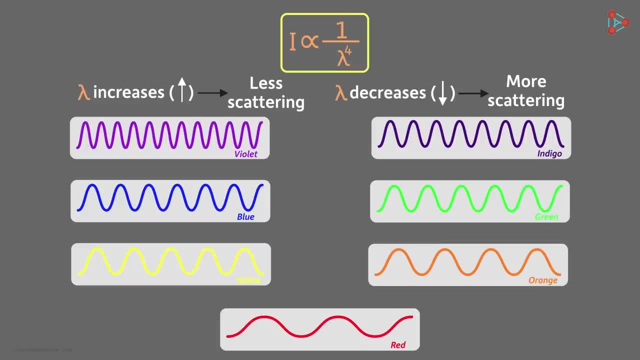 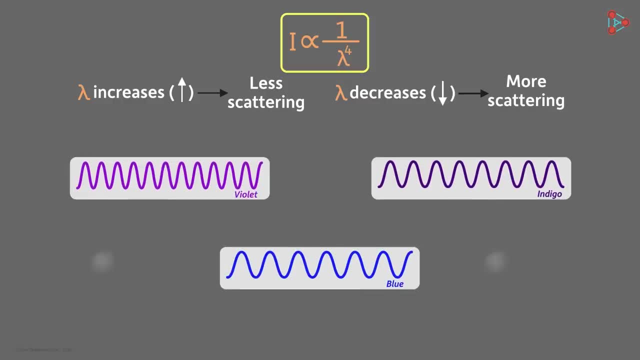 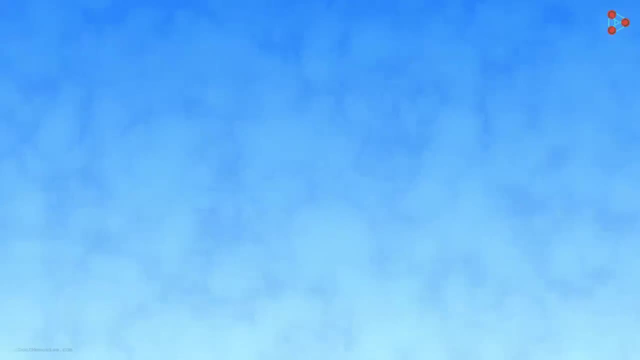 the most. Yes, the light of the colour corresponding to the smallest wavelength will be scattered the most. So blue, indigo and violet light will be scattered most by these molecules of air. And when this light travels to our eyes, the sky appears blue to us. 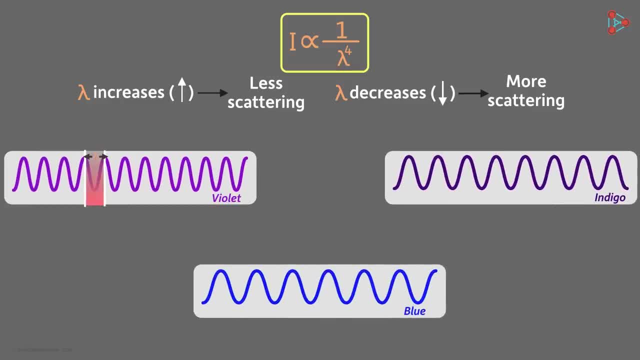 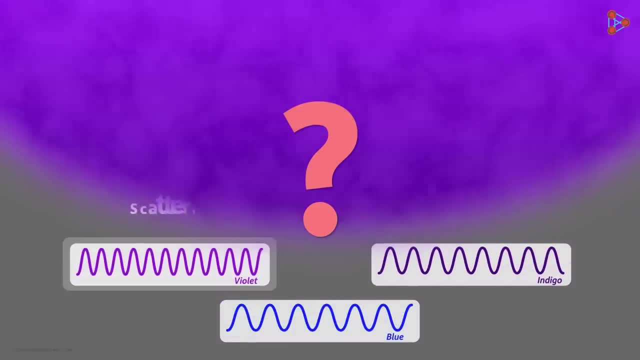 But wait, The violet light has the smallest wavelength, Then why doesn't the sky appear violet, or even indigo, for that matter? It is true that the sky scatters the violet light more than the blue light. However, we don't see violet sky, do we?